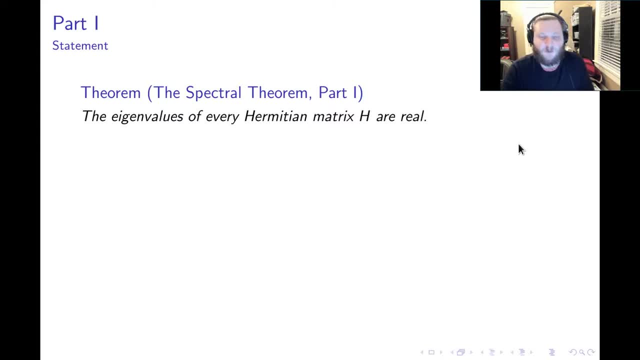 So let's see the proof. I think it's actually worth walking through the proof here. If for no other reason, it's a nice exercise in understanding inner products. So here's how the proof is going to go. So the Hermitian matrix we're dealing with is called H here. 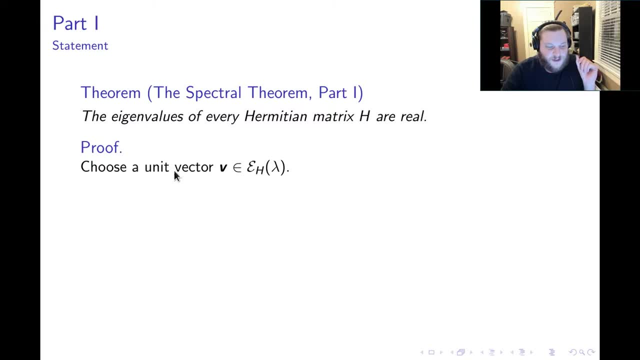 So to start the proof, we're going to start with a unit-threaded vector V in the eigenspace of H, where the eigenvalue we're studying here is lambda. Now our goal here is to argue that lambda is a real number. So how are we going to do that? 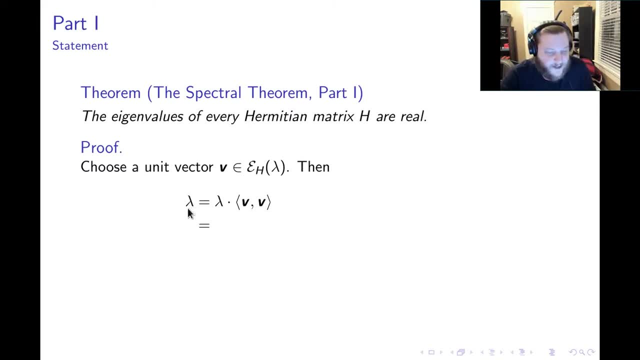 Well, the first thing we're going to say is that lambda is the same thing as lambda times the inner product of V with itself. Now, why is that the case? Well, by construction here, we're choosing V to be a unit vector, and the inner product of any vector with itself is always equal to its length squared. 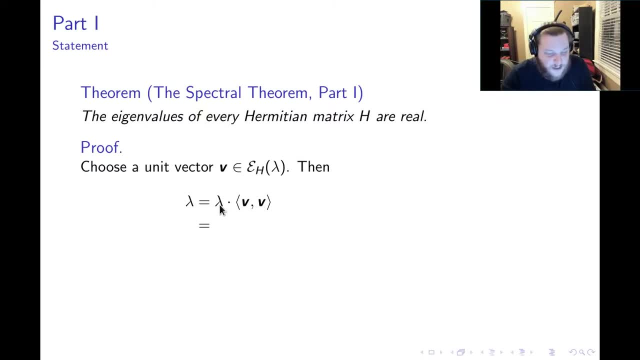 which is 1 here. So lambda is certainly equal to lambda times 1.. Great, Now we're going to push lambda into the second slot of our inner product. Remember that we can always push a scalar into an inner product. If we push it into the second slot, we don't have to change the number. 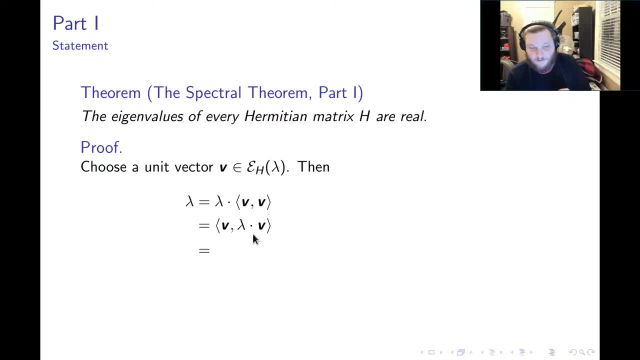 but if we push it the first slot, we have to conjugate the number. Now we see we're looking at the inner product of V with lambda times V. but the whole point of V here is that V is an eigenvector of H corresponding to the eigenvalue lambda, so lambda times V. 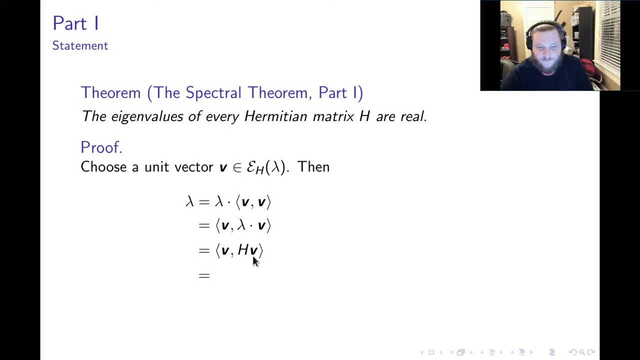 is the same thing as H times V. Now we're looking at the inner product of V with H times V. but remember the adjoint formula for inner products says that matrices can bounce back and forth inside of an inner product, except every time we move a matrix from one side to the other we have to take its conjugate. 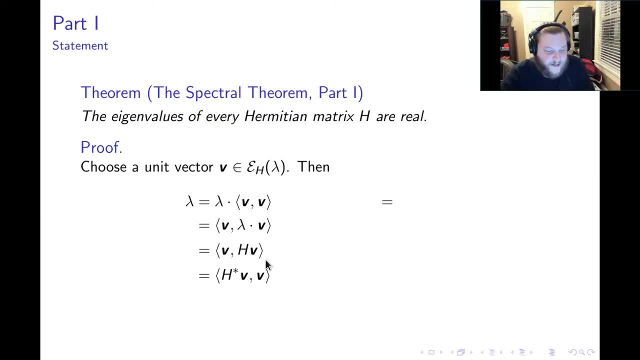 transpose. So we can move H from the right to the left here by taking its conjugate transpose. But now the whole point of H in this setup here is that H is Hermitian, which means it's common and it's conjugate. So the whole point of H is that H is Hermitian, which means it's. 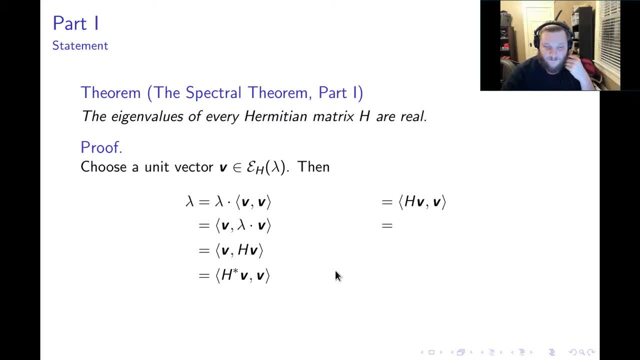 conjugate. So the whole point of H in this setup here is that H is Hermitian, which means it's conjugate, transpose equals itself. So now we're looking at h times v, inner product with v. Well, h times v, we already know, is equal to lambda times v. So we've gone through all this. 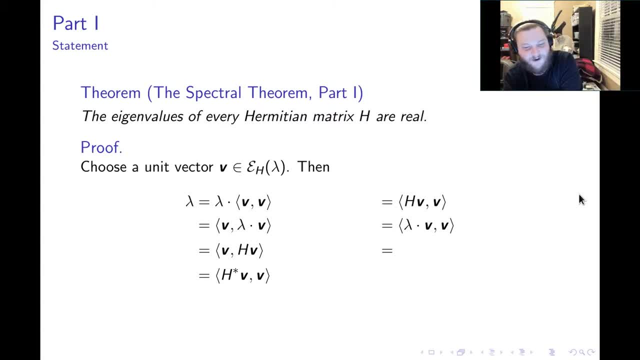 trouble to move lambda from the right-hand side of our inner product to the left-hand side. And now we know that we can factor out scalars from the first slot of an inner product, but when we do that, it's not the scalar that factors out, it's conjugate that factors out. 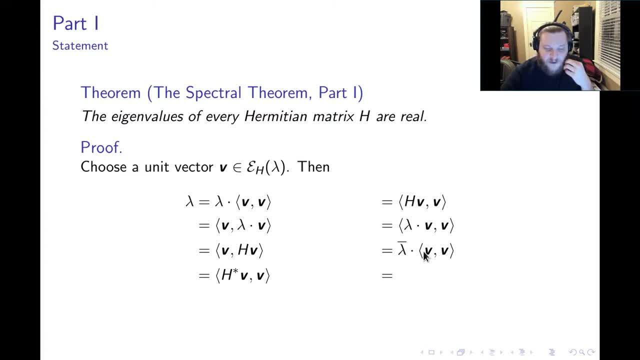 And now we're looking at the conjugate of lambda multiplied by v, inner product with v. but again, v in this situation is a unit vector, so the inner product of v with itself is equal to 1.. So ultimately we're just looking at the conjugate of lambda here, So there's several. 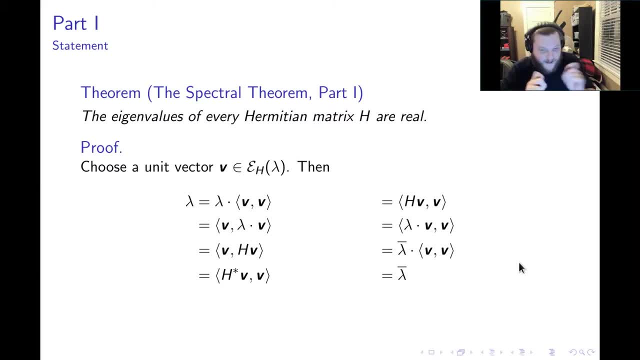 equalities that we went through. but if we pay attention to start and finish, we see that what we've set up gives us lambda at the beginning, which is equal to the conjugate of lambda, And the only numbers that are equal to their own conjugates are real numbers. 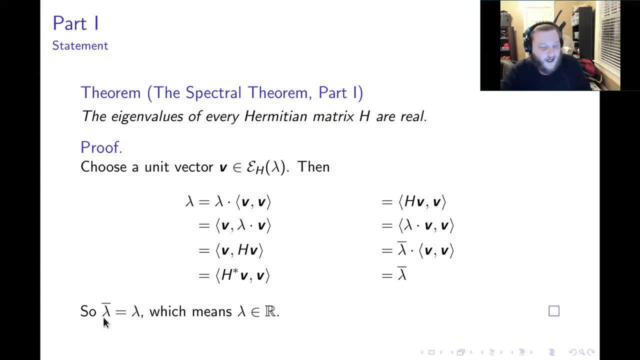 So this argument tells us that the conjugate of lambda equals lambda, which means that lambda was a real number to begin with. So we started with an arbitrary eigenvalue of this Hermitian matrix, And this argument tells us that that eigenvalue is guaranteed to be a real number. 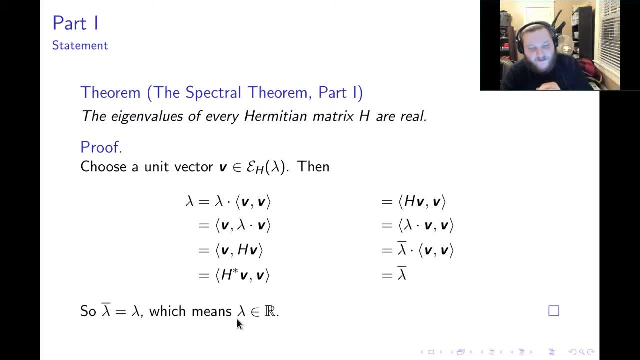 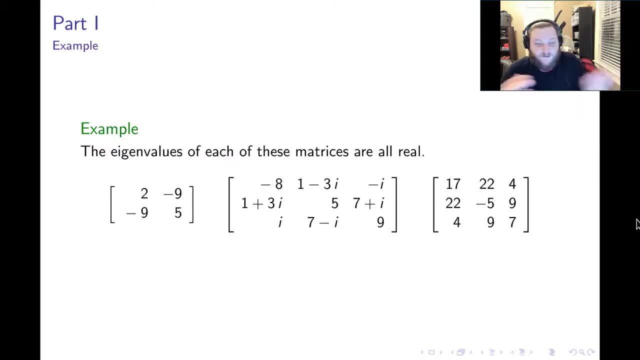 So this is the first part of the spectral theorem. Any eigenvalue of a Hermitian matrix is guaranteed to be a real number. So let's just briefly apply this concept. This the first part of the spectrum. the spectral theorem immediately tells me: 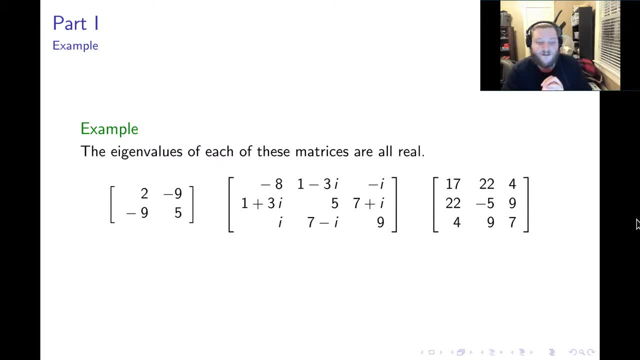 that the eigenvalues of each one of these three matrices are all real. Why are the eigenvalues of my first matrix here real numbers? Well, keep in mind, I'm not telling you what the eigenvalues are. I'm simply saying that I can use the theorem we just proved to argue that the eigenvalues of